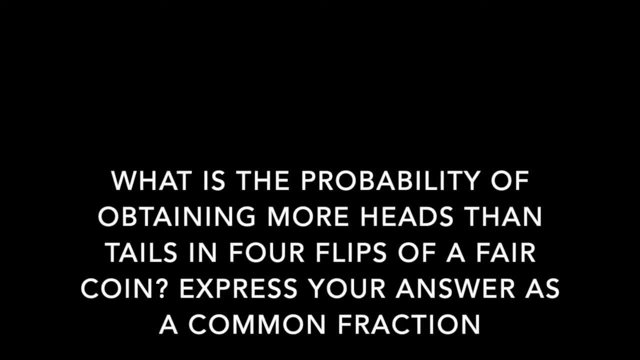 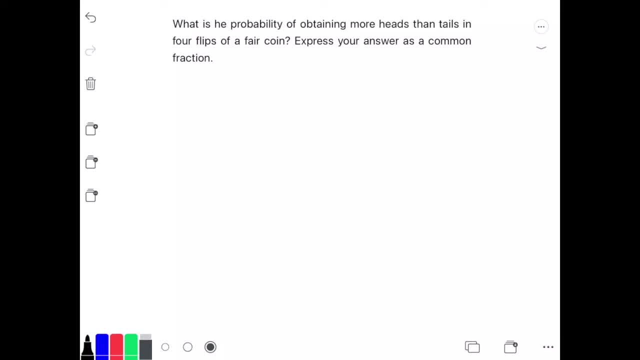 The question is asking for the probability of obtaining more heads than tails on four flips of a coin. so we can start by finding the total outcomes And if we flip the coin four times- for the first flip, second flip, third flip and the fourth flip- we have two outcomes for each flip and that's heads and tails. 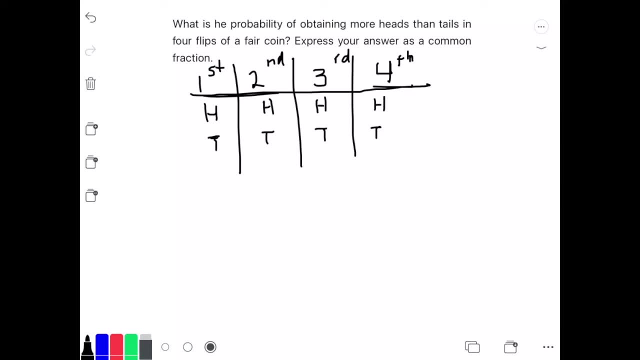 And then we compare the heads and tails, So we get two outcomes. and then we compare the tails and heads and tails and tails, so we get two more outcomes and we can multiply them because they're independent events. And then we repeat the step for the third flip and then the fourth flip. 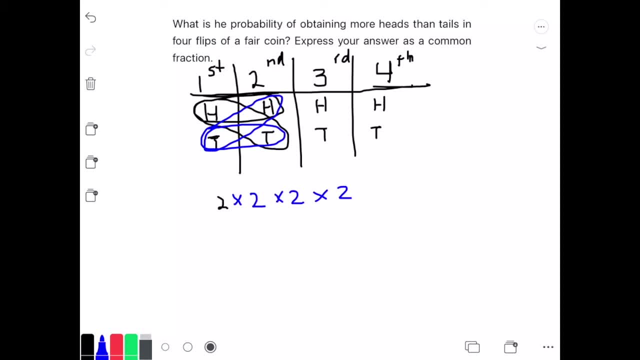 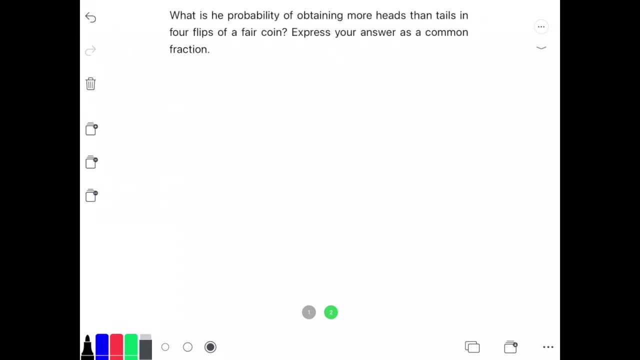 So we have two times two times two, And that's sixteen. So we have sixteen total outcomes, And then the probability of obtaining more heads than tails. We can list the combinations for heads and tails and we get heads, heads, heads, heads. 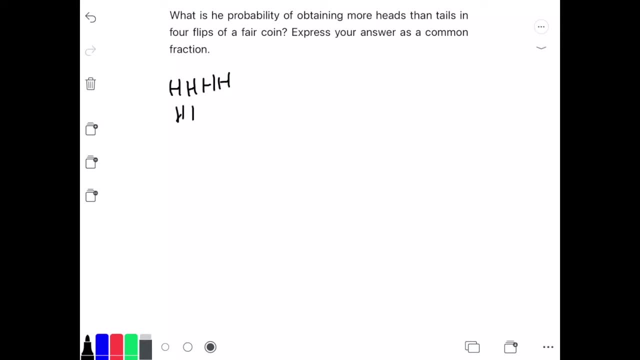 And then heads, heads, heads, tails Heads, heads tails heads. And then heads, heads, tails, tails, Heads, tails heads, heads, Heads, tails, heads, tails, Heads, tails, tails heads. 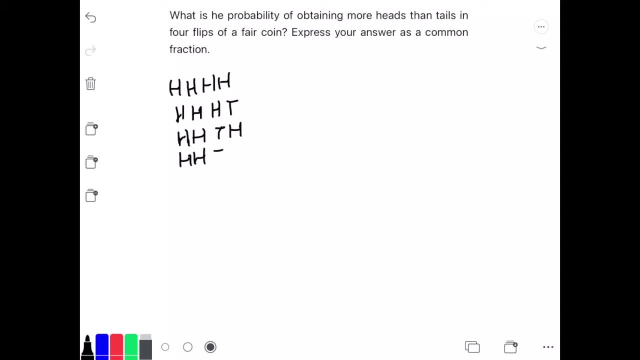 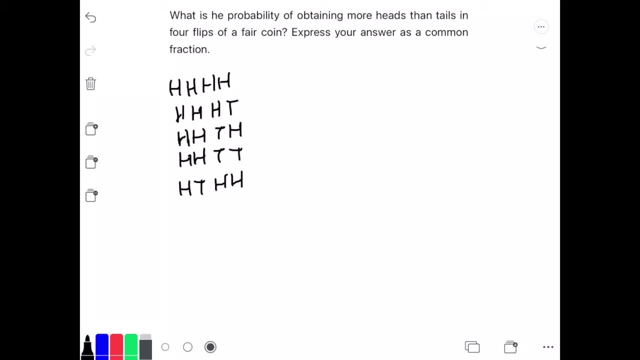 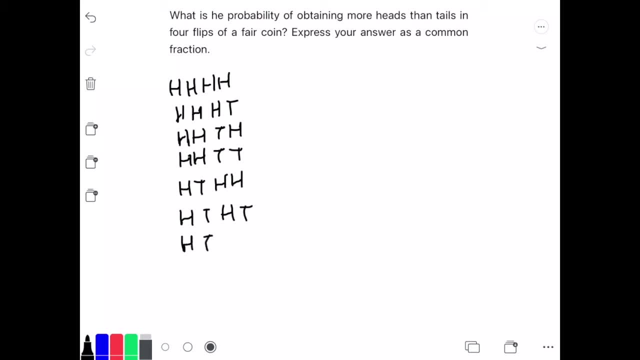 Heads, tails, tails, tails, heads, tails, tails, heads, and then we have tails, heads, heads, heads, and then we can circle the combinations that have more heads than tails. so we can circle the heads, heads.